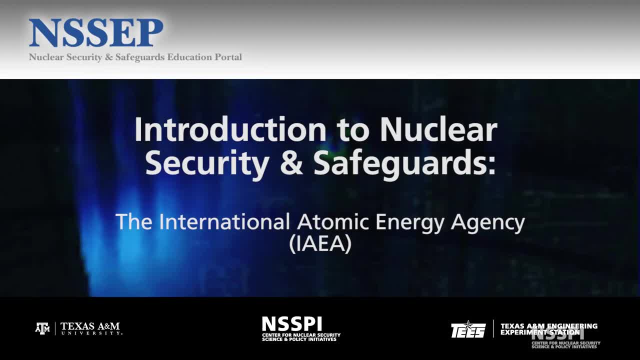 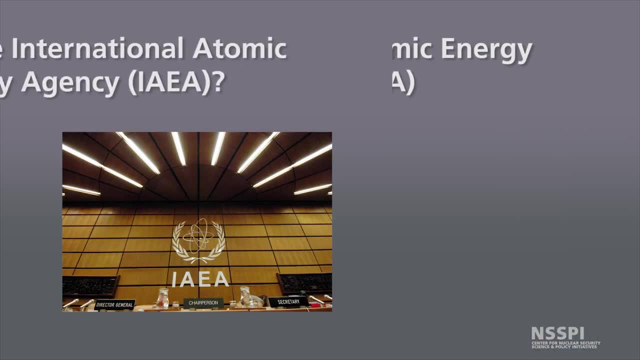 In this section we're going to discuss the International Atomic Energy Agency, the IAEA. So what is the International Atomic Energy Agency? Well, to understand that first we have to go back to December 8, 1953, was when US President Eisenhower gave his famous 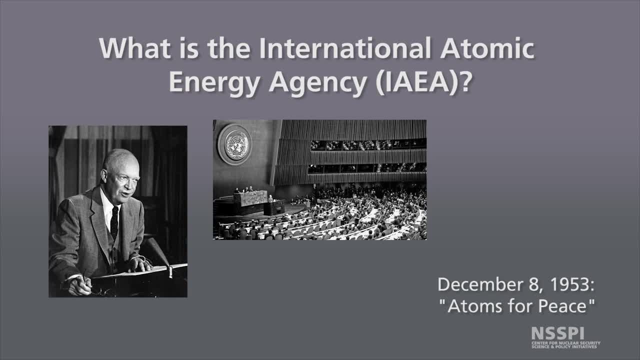 Atoms for Peace address to the UN General Assembly. In this address he talked about promoting the benefits of civilian nuclear power throughout the world through the Atoms for Peace Initiative. Then, in October of 1956, the IAEA statute was unanimously approved. 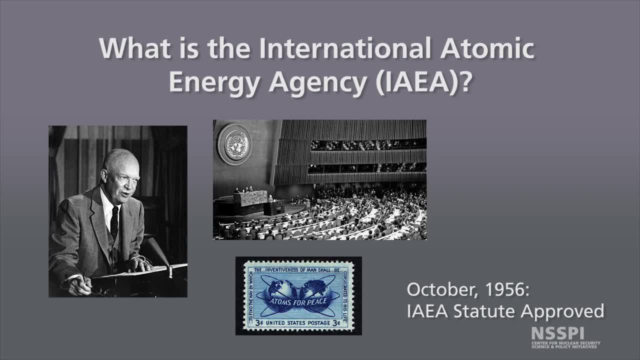 by 81 nations within the UN. Since then the IAEA has worked to promote the ideals discussed in Eisenhower's Atoms for Peace Initiative. So now it is worthwhile to discuss the International Atomic Energy Agency, the IAEA, and the US. 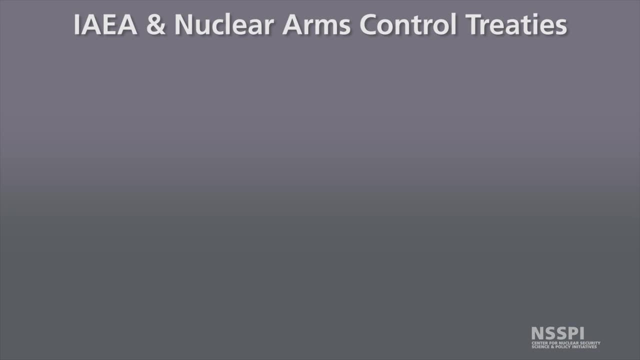 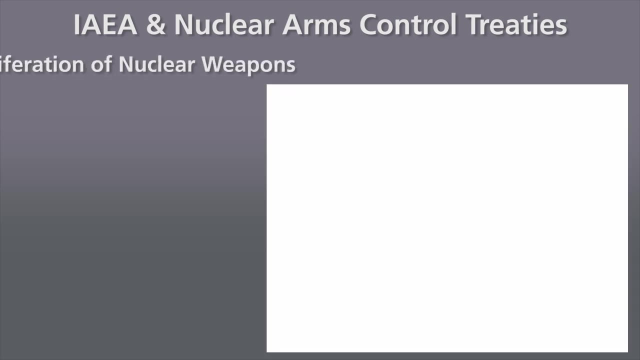 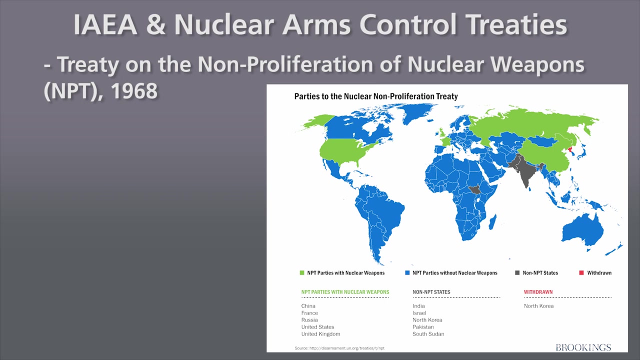 National Atomic Energy Agency discuss the role of the IAEA in relation to several nuclear arms control treaties. The first and most important nuclear arms control treaty is the Treaty on the Non-Proliferation of Nuclear Weapons, the NPT, which was initiated in 1968. 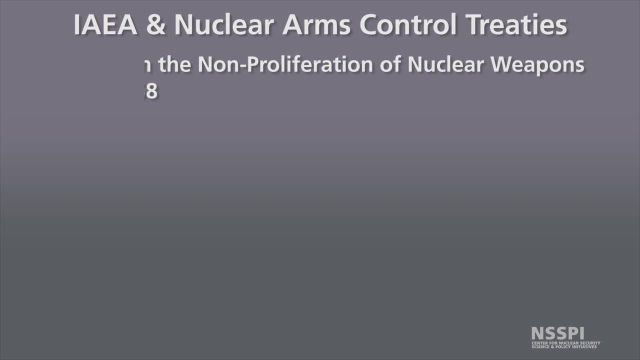 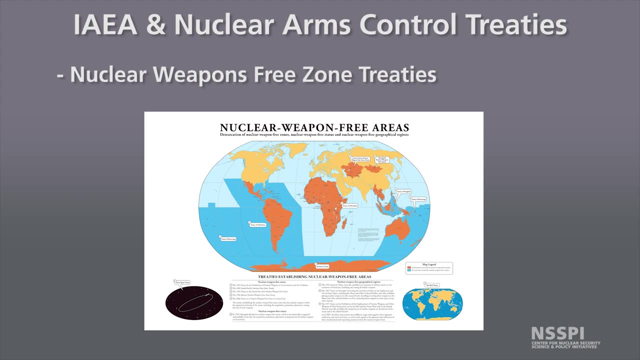 In addition to the NPT, there are several nuclear weapons free zone treaties, and the basic idea of these is that there's a region of specific states in the world that decide that they don't want nuclear weapons in any of those regional states or anywhere in their 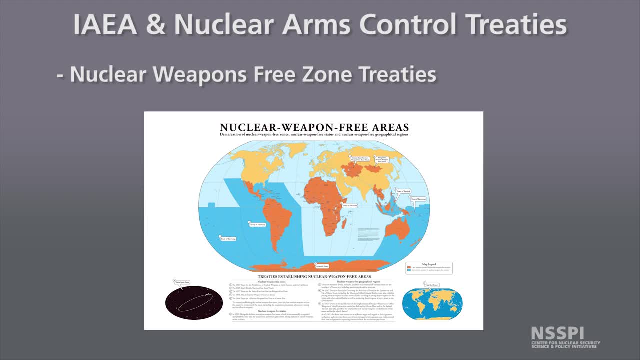 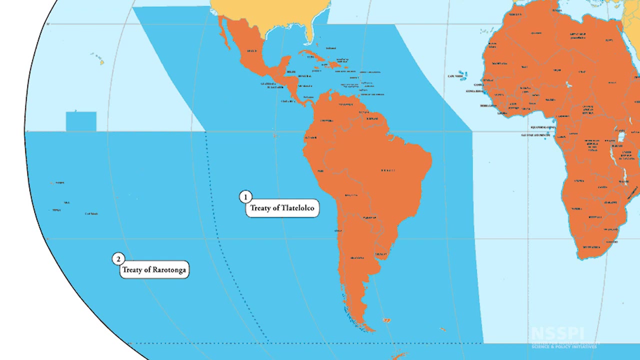 region, whether it's from one of the regional states or from some state outside of the region covered by the treaty. And there are five of those treaties: the Treaty of Latiloco, which covers Latin America and the Caribbean. This was signed in 1967.. 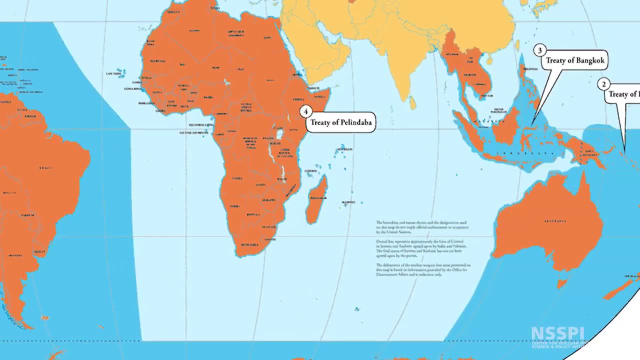 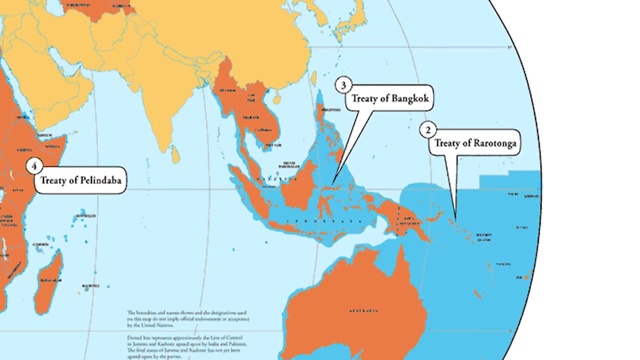 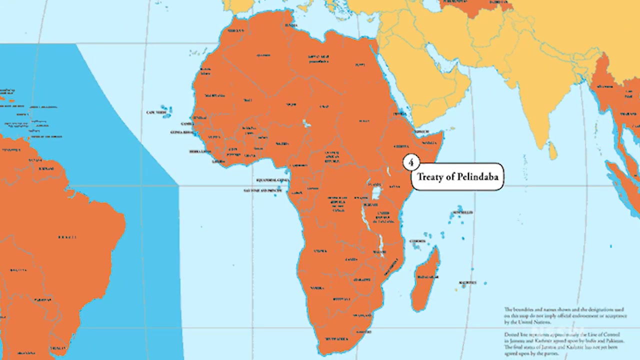 And then the Treaty of Rarotonga, covering the South Pacific, in 1985.. The Treaty of Bangkok, which covers Southeast Asia, in 1995.. The Treaty of Palindaba, which covers Africa, and this was signed in 1996..